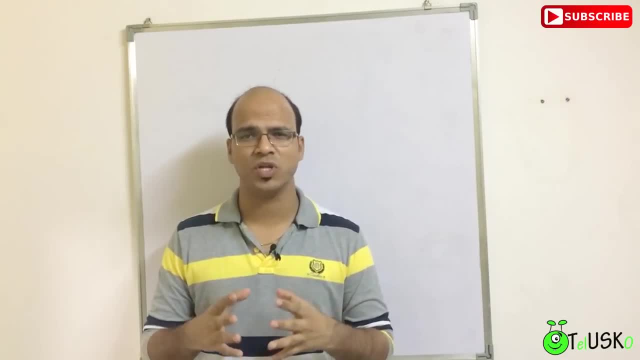 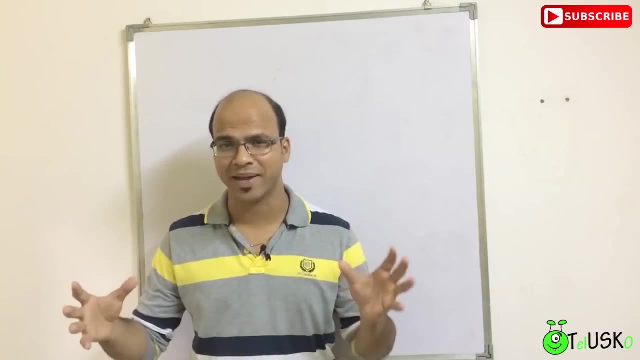 welcome aliens. this is ravin reddy from talisco learnings, and in this video we'll talk about builder design pattern. so we have already already discussed about design patterns. right, so we have three different design patterns. we have creation design pattern, we have structural and then we have 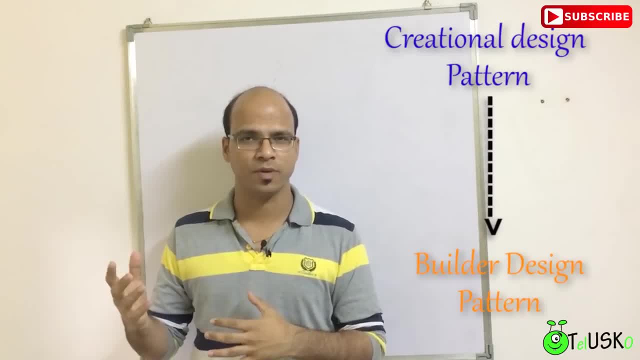 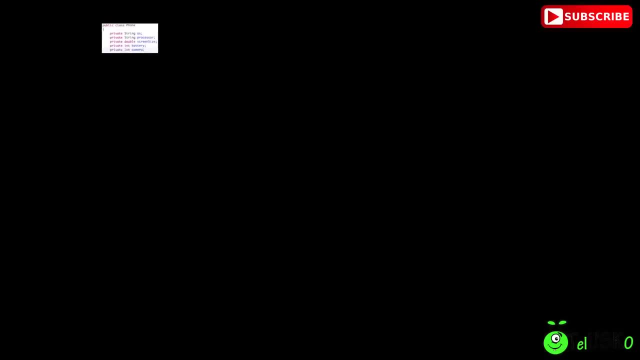 behavioral builder pattern is a part of creational, because it will be helpful when you create an object. now, just to explain this, let's go for an example. so let's say we have this phone class in which you have five variables. so we have os, we have battery, we have a camera, we have processor. 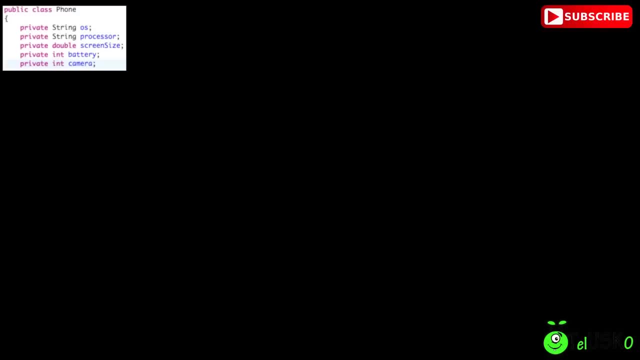 and what we have: screen size. so let's say we have these five variables. now, in order to create object of this phone, we require those five values. right, so we can set the values with the help of setters or we can use constructor way. right now, let's say i'm using constructor here, so in my constructor, 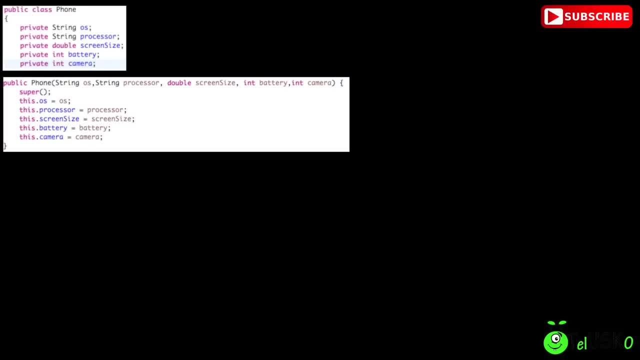 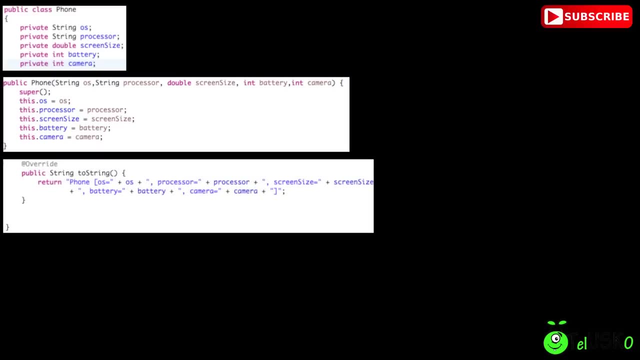 i have five parameters, so i'm using a parameterized constructor. right, so that that's a. that's what the class we have here. we also have a parameterized constructor, so that's what we have here. we also have a two string method, so that when we print the object, we'll get that method. right now i want to. 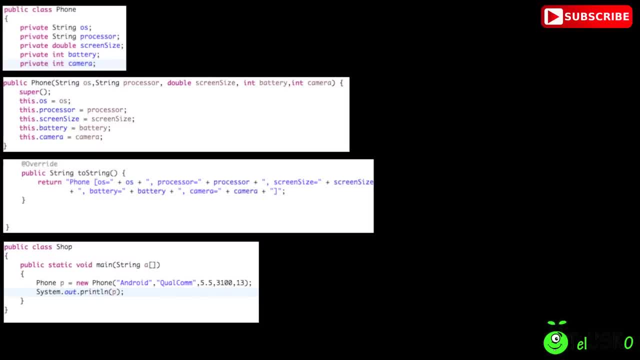 create object of phone here. so we have a class which is shop and inside that you have a main method. so what we'll do is we'll try to create object of phone here now, how to get object of phone. so we'll say phone p and we have to say new phone. right, we have to pass five parameters. 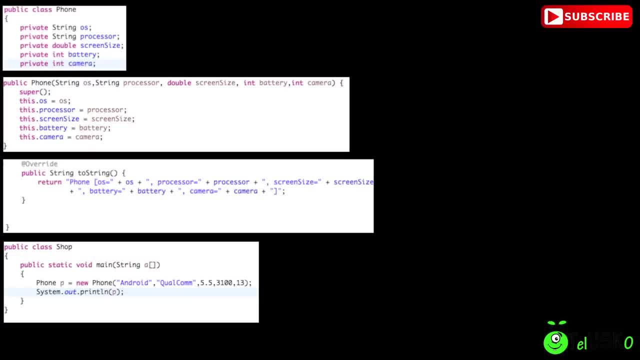 and that's the question: what are the parameters we have to pass here and within which sequence? so i have to pass os, i have to, i have to pass battery, have to pass screen size. so we have to pass all those parameters right. so the concerns are we: 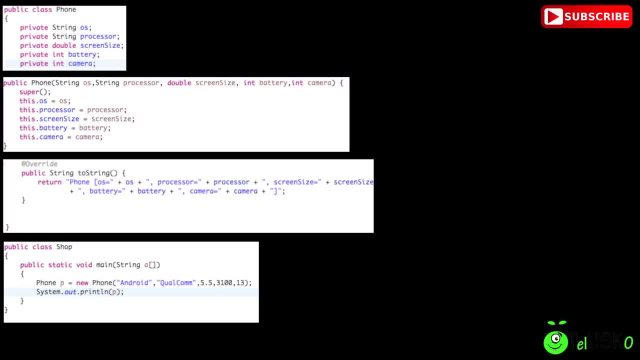 have to. we have to pass five parameters we have. we should remember the sequence of the parameters in which sequence you have to send. so that's the problem here, and maybe i don't want to set all the parameters. i want to set only the os, i want only i. i want to set only the ram or not ram. but 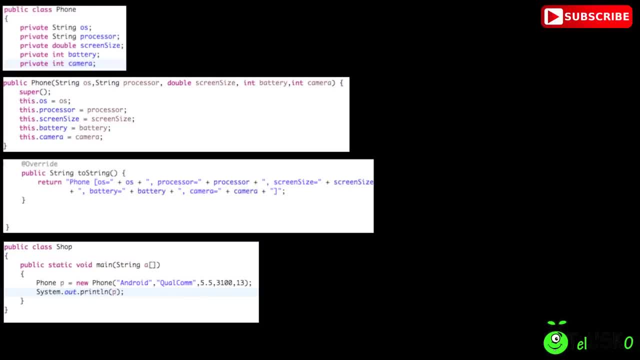 but maybe size. i don't want to set all the parameters. example, if you want to buy a phone, you check all the things, right, you check which phone you're buying, maybe os, you check which, what's the screen size, you check for the battery, but let's say there are some people that are not. 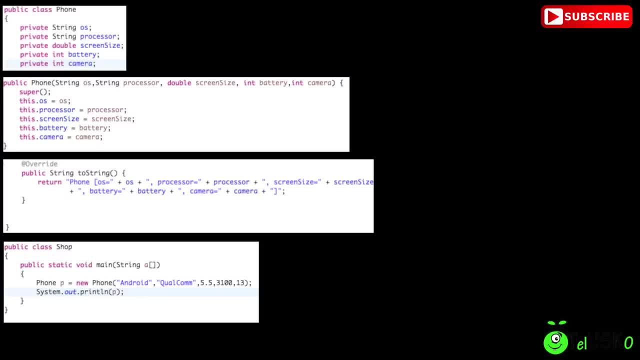 concerned about all those features. they're only concerned about the phone. they want android phone. doesn't matter which android phone they want, it depends upon the budget, right? so they want an android phone. there are some people that doesn't. this doesn't matter which os they have, they want. 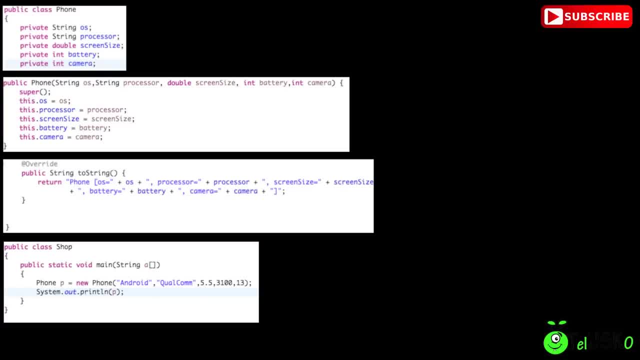 a phone to call someone. they want a smartphone. doesn't matter which os they have- maybe android, maybe ios or windows- they want a smartphone, right. so in this scenario we cannot pass all the parameters right, so there's a problem here. so first, we don't want to set all the parameters. 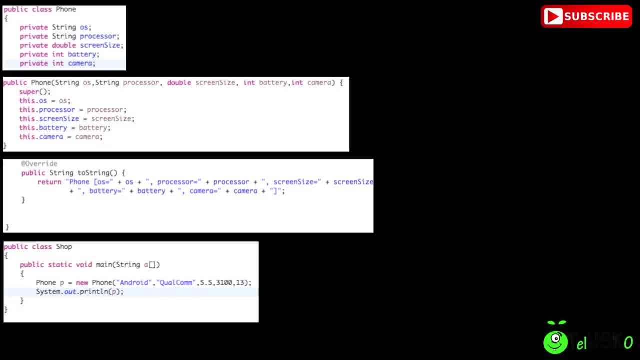 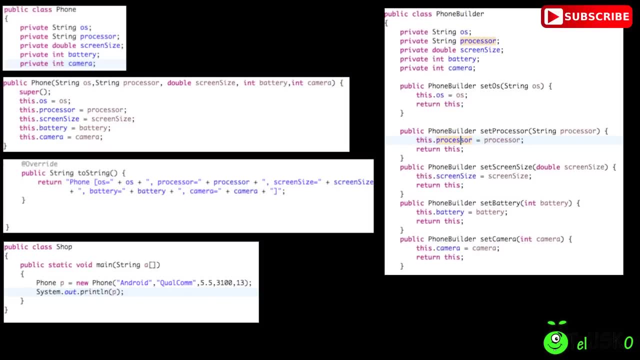 second, even if you want to pass all the parameters, you should know the sequence of the constructor, right? so that's why we use design or say builder, design pattern here. now how it works. so just imagine we have a class here which is builder, a phone builder, and now in this class we'll be 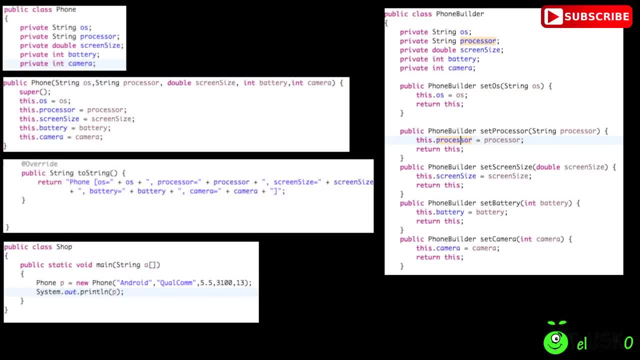 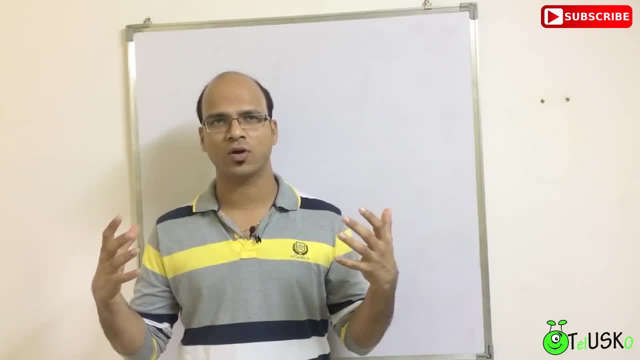 having all the variables which are there in the phone class itself, and then we'll be having some setters. now the not just to explain. you can see that we have a setter which is a setter which is custom, but what we're going to do is we're going to set up a setter to display the with the. 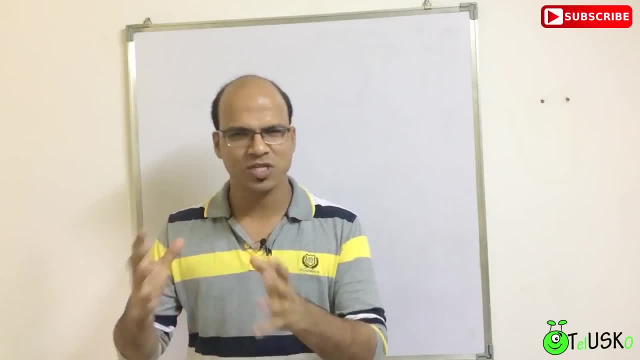 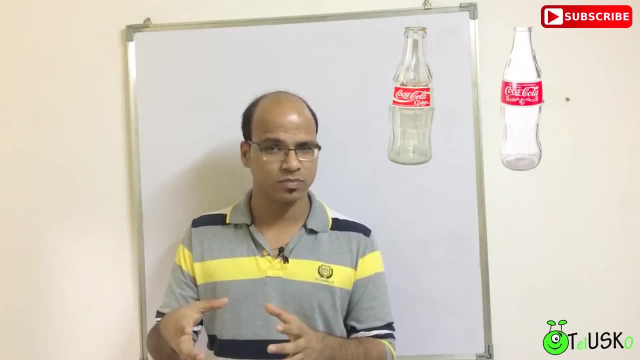 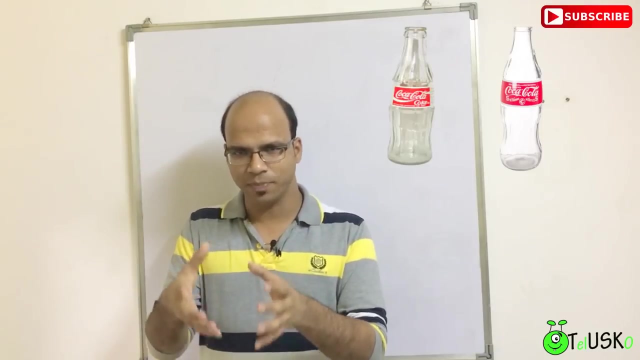 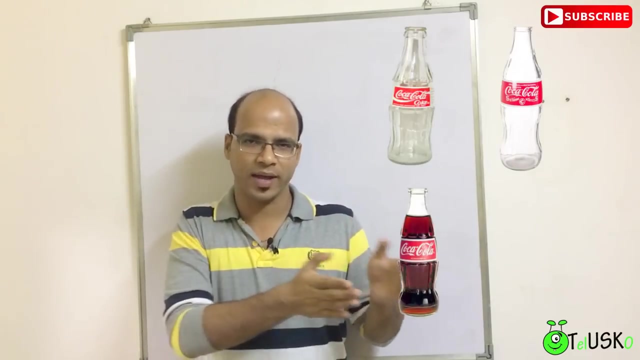 set with a vr file. this way, just to say that it's actually going to display the lineup box, not just the unique mod 's. the own advantages of this is that you don't have to send basically any kind of custom layout. all right, let's move on to level one here. so you see that you take this maximize bitch. 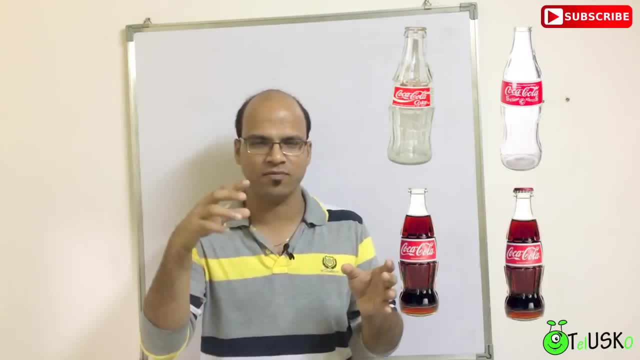 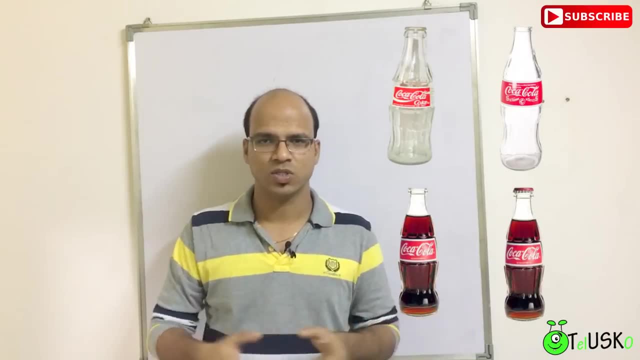 is that all in this is have to provide. we have to attach a cap there. so we have, we are applying a cap, the same bottle will go ahead and then we'll be applying a label, right, so that's how it works. so this: we are providing the same object as an input and the output will be the same object, right? so if you're passing object, 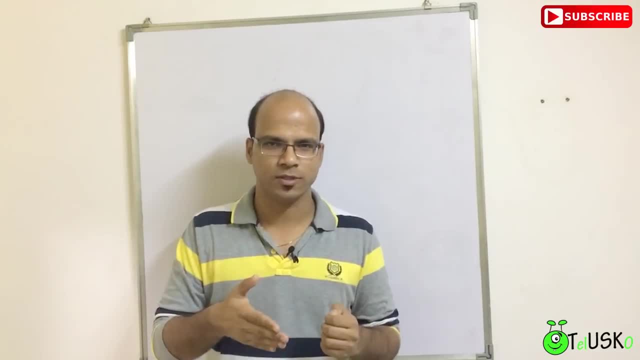 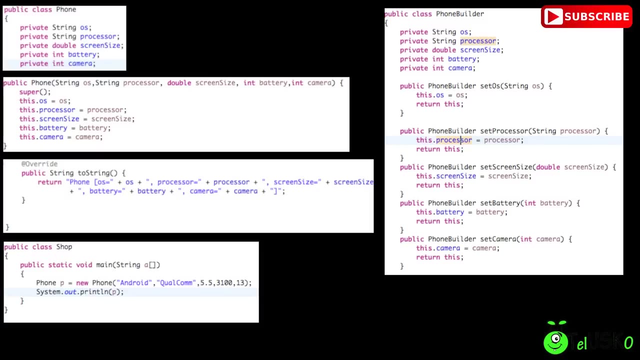 a it goes inside the same objects comes out. so that is builder pattern. so how this phone builder will works in every center. what we have here is: in every sector it returns the object of phone builder itself, okay. so that's why we say: return this right, so we are passing the same object and 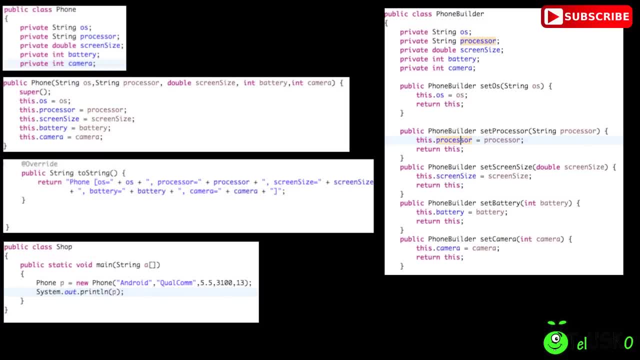 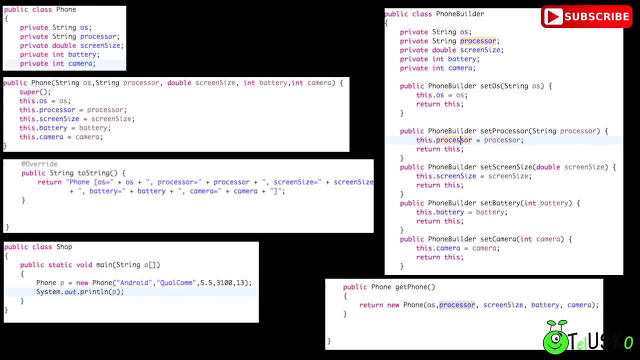 we are, we are, we are changing the values and we are taking out the same object- right, that is phone builder- and at the end we have a method which is get phone, and this get phone will give you object of phone- awesome, right, and the advantage will be now inside your shop class. what you can simply do.